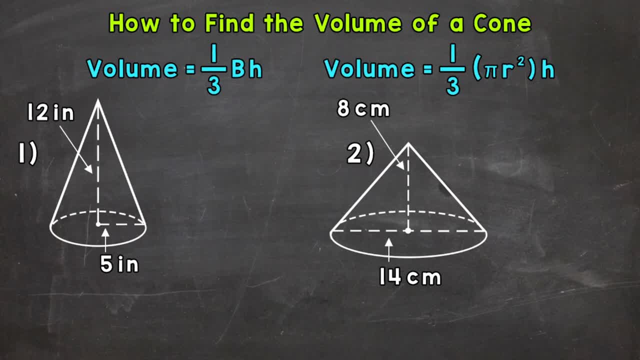 formula at the top left of the screen. But since the base of a cone is a circle, we can input the formula for the area of a circle into our volume formula to make it more specific. So, the formula to the right at the top of the screen, We have one-third times the area of the circular base. 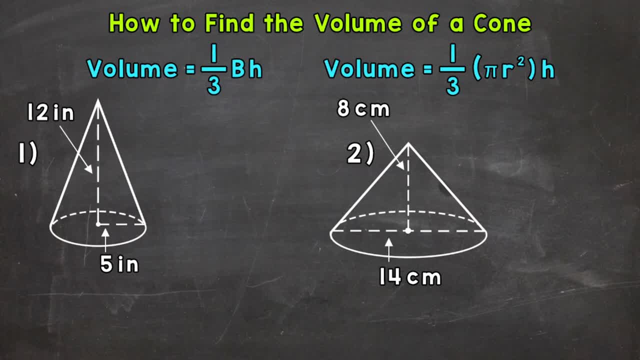 pi r squared times the height. Now we'll talk about why we multiply by one-third after we finish numbering, But first let's look at the formula for the volume of a cone Number one: Knowing why we do this will give us a better understanding of the formula. So let's 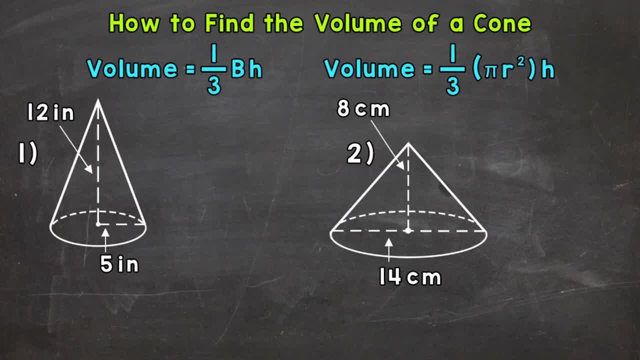 jump into number one, where we have a cone with a base radius of 5 inches and then a height of 12 inches, And the first thing that we need to do is write out our formula. So volume equals one-third times the area of our base. so pi? r squared, since we have a circular base, and then times the height. 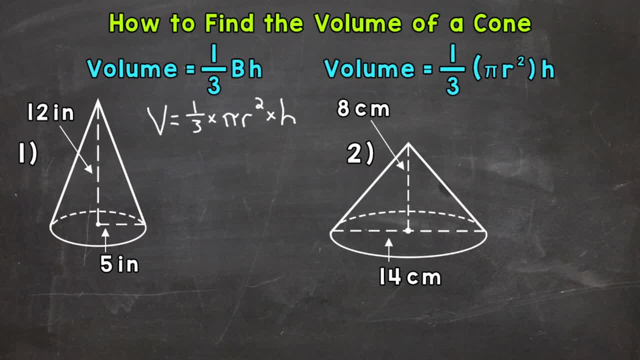 Now I wrote out the formula a little different than how it's written at the top of the screen. That's okay, because I'm still multiplying one-third times the area of the base, times the height. It doesn't matter how you represent the multiplication symbols or parentheses. 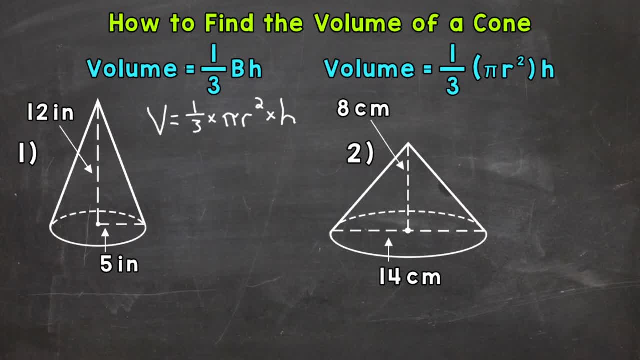 as long as you're multiplying one-third times the area of the base times the height. So once we have our formula written we can plug in our radius and height. So we have: volume equals one-third times pi, our radius of 5, squared times the height, which is 12.. 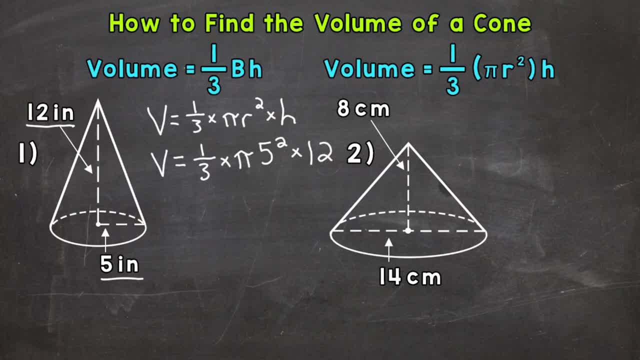 Now, at this point we're ready to solve, So we can plug that into a calculator and we'll have the volume of that cylinder. I'm going to break it down or simplify it a little further, though, until we get it to the right value. So let's go ahead and do that. So let's go ahead and do that. 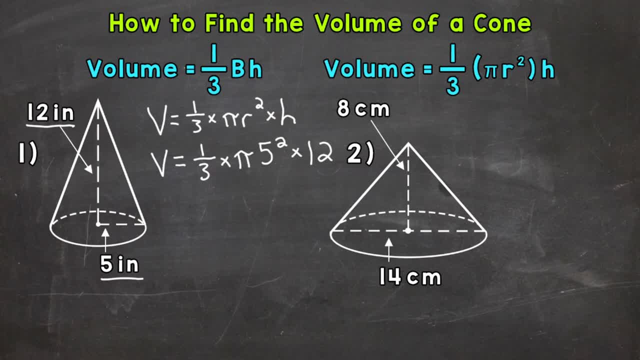 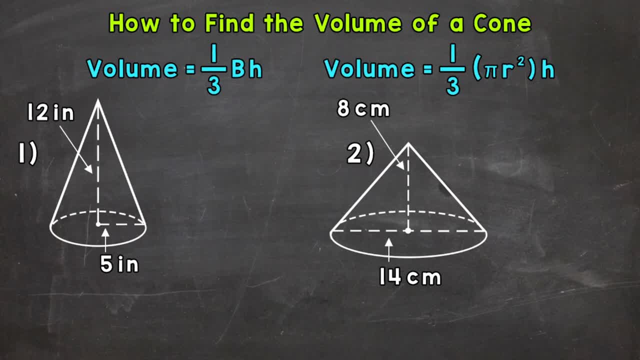 formula at the top left of the screen. But since the base of a cone is a circle, we can input the formula for the area of a circle into our volume formula to make it more specific. So, the formula to the right at the top of the screen, We have one-third times the area of the circular base. 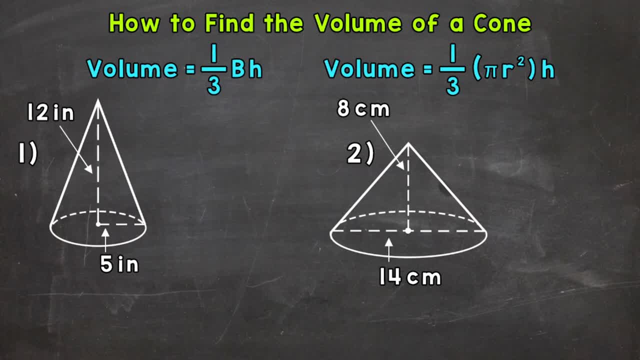 pi r squared times the height. Now we'll talk about why we multiply by one-third after we finish numbering, But first let's look at the formula for the volume of a cone Number one: Knowing why we do this will give us a better understanding of the formula. So let's 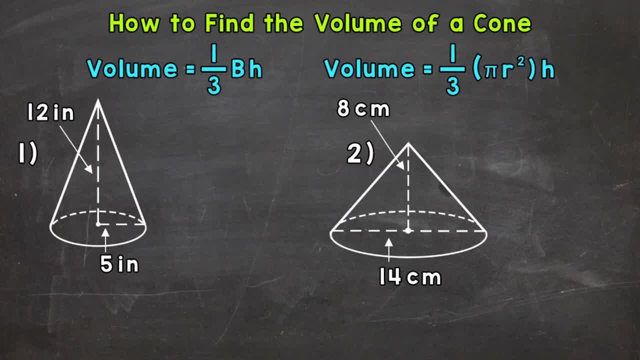 jump into number one, where we have a cone with a base radius of 5 inches and then a height of 12 inches, And the first thing that we need to do is write out our formula. So volume equals one-third times the area of our base. so pi? r squared, since we have a circular base, and then times the height. 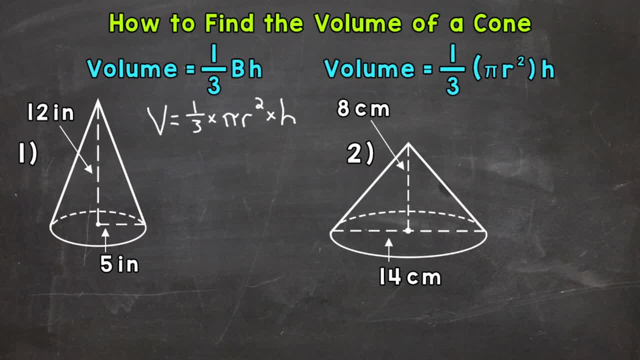 Now I wrote out the formula a little different than how it's written at the top of the screen. That's okay, because I'm still multiplying one-third times the area of the base, times the height. It doesn't matter how you represent the multiplication symbols or parentheses. 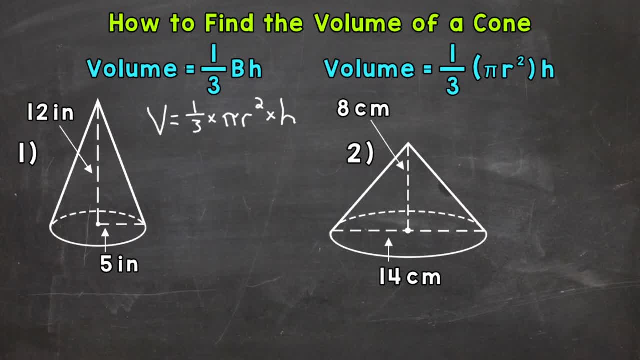 as long as you're multiplying one-third times the area of the base times the height. So once we have our formula written we can plug in our radius and height. So we have: volume equals one-third times pi, our radius of 5, squared times the height, which is 12.. 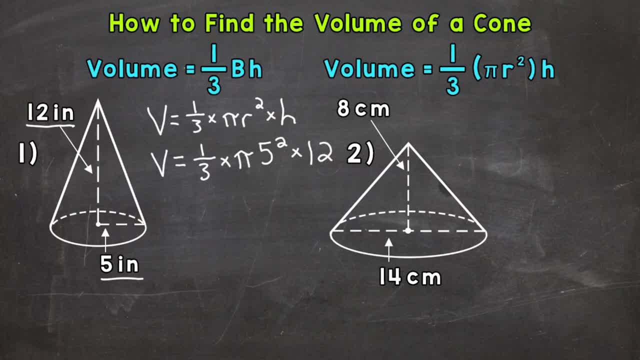 Now, at this point we're ready to solve, So we can plug that into a calculator and we'll have the volume of that cylinder. I'm going to break it down or simplify it a little further, though, until we get it to the right value. So let's go ahead and do that. So let's go ahead and do that. 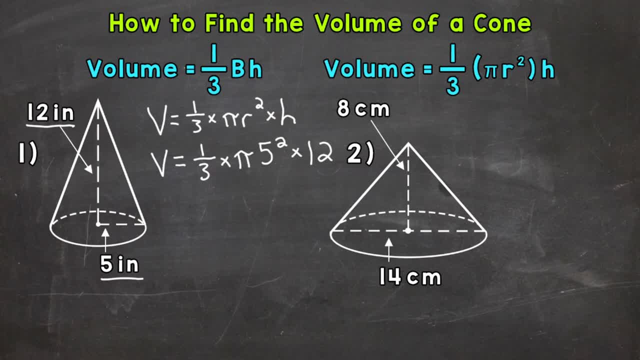 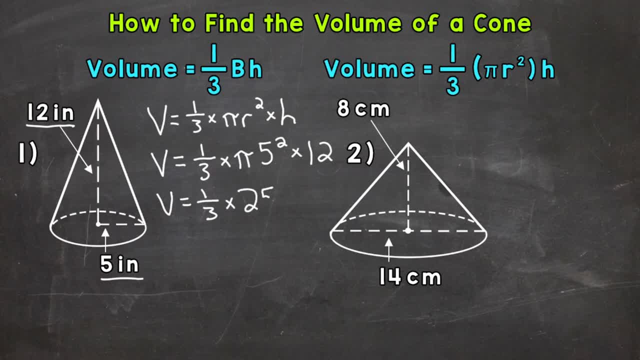 that gives us 25 times pi, 25 pi times 12.. Now I put the 25 in front of the pi symbol because we simplified the area of the base and now we have it in terms of pi And, typically speaking, you'll put a number in front of pi when multiplying a number by pi. So we are ready to move forward. 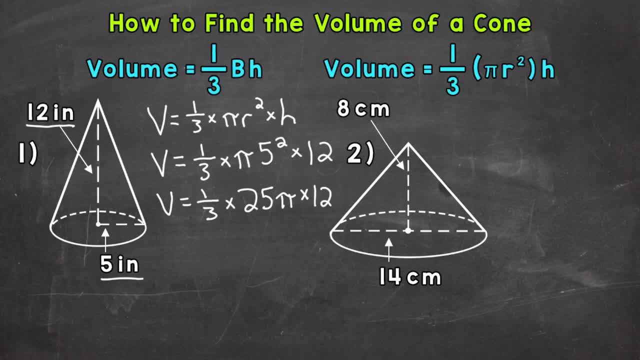 here and we have a couple of different ways we can do the next step. So one way: we can cross cancel, or multiply one-third and 12, or we can do 25 times 12.. I'm going to do 25 times 12 and that. 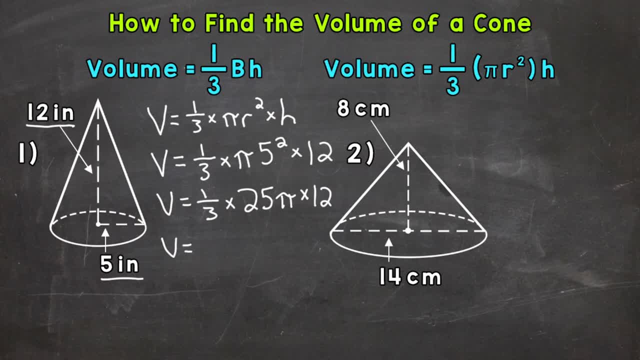 gives us 25 times 12.. So we have a couple of different ways we can do the next step. So one way: volume equals one-third times well, 25 times 12 is 300, and pi. So one-third times 300, pi. Now we 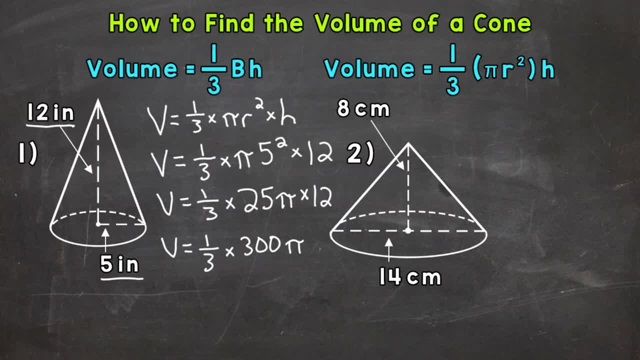 have one-third times 300, or one-third of 300. That will give us 100 pi, And that's our answer in terms of pi. Now I'm going to calculate the exact volume by multiplying 100 times pi And I'm going to use 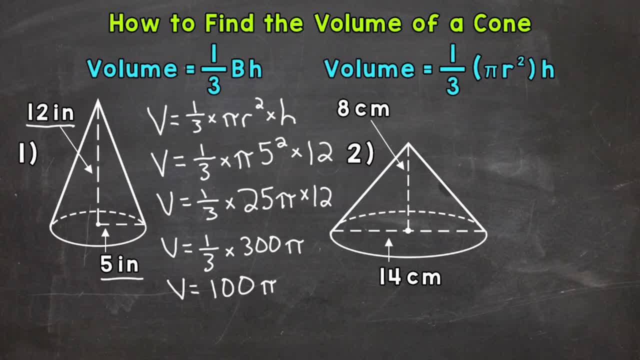 the pi button on a calculator. Now it's common practice to also use the rounded version of pi 3.14.. Both are correct, but know that answers will vary slightly depending on if you use the rounded version 3.14, or the pi button on a calculator. So again, I'm going to use the pi. 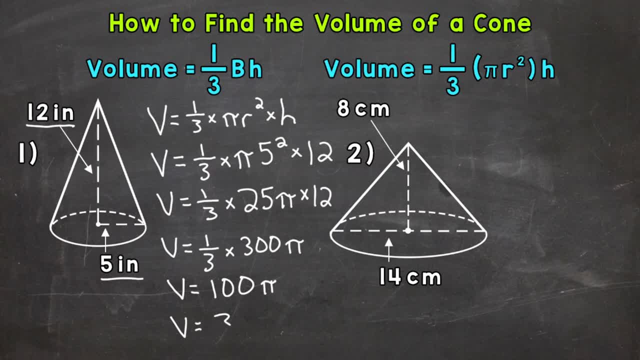 button And we get volume equals 314.. And I'm going to round the decimal to the hundredths place. So we get 16 hundredths So 314, and 16 hundredths or 0.16.. And this is cubic inches, because we're talking. 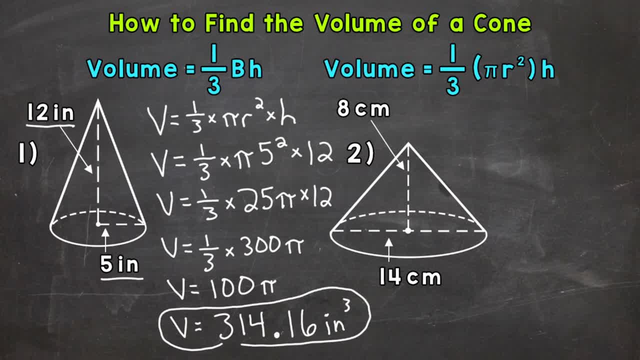 volume. So that's our final answer right there. So I want to explain why we multiply everything by one-third times pi. So I'm going to use the pi button on a calculator And I'm going to use the pi button on a calculator. 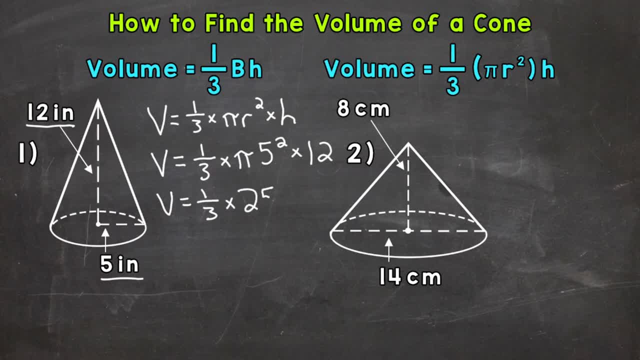 that gives us 25 times pi, 25 pi times 12.. Now I put the 25 in front of the pi symbol because we simplified the area of the base and now we have it in terms of pi And, typically speaking, you'll put a number in front of pi when multiplying a number by pi. So we are ready to move forward. 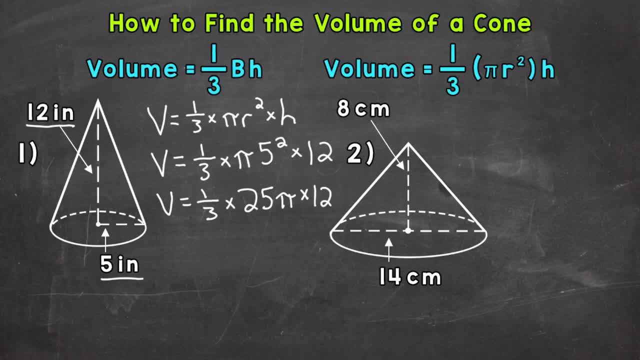 here and we have a couple of different ways we can do the next step. So one way: we can cross cancel, or multiply one-third and 12, or we can do 25 times 12.. I'm going to do 25 times 12 and that. 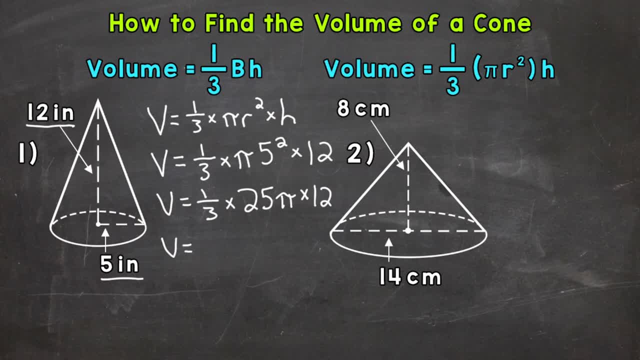 gives us 25 times 12.. So we have a couple of different ways we can do the next step. So one way: volume equals one-third times well, 25 times 12 is 300, and pi. So one-third times 300, pi. Now we 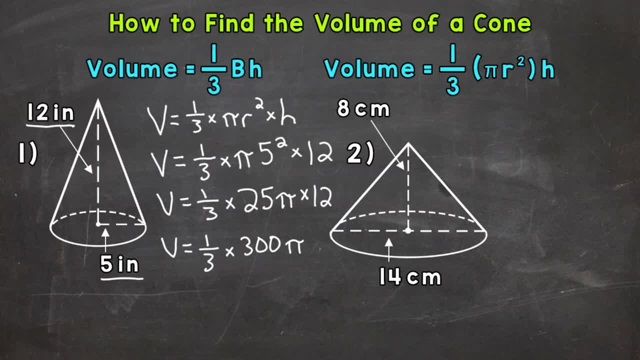 have one-third times 300, or one-third of 300. That will give us 100 pi, And that's our answer in terms of pi. Now I'm going to calculate the exact volume by multiplying 100 times pi And I'm going to use 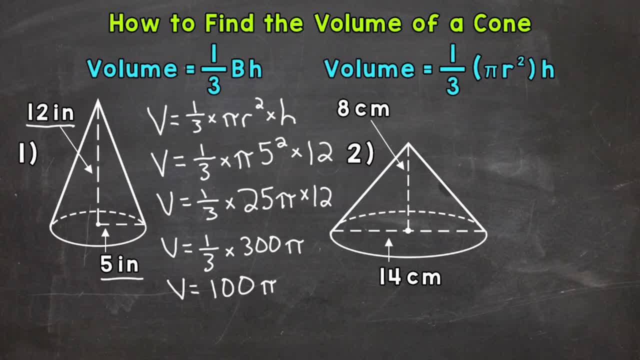 the pi button on a calculator. Now it's common practice to also use the rounded version of pi 3.14.. Both are correct, but know that answers will vary slightly depending on if you use the rounded version 3.14, or the pi button on a calculator. So again, I'm going to use the pi. 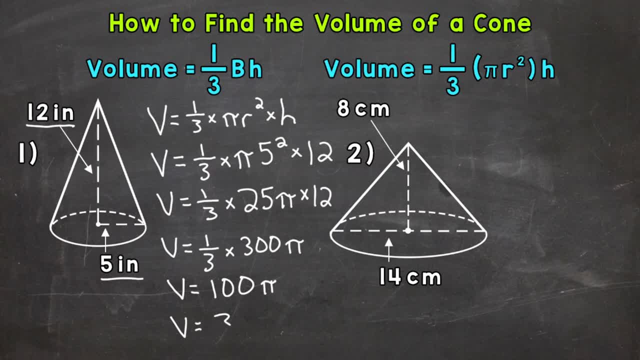 button And we get volume equals 314.. And I'm going to round the decimal to the hundredths place. So we get 16 hundredths So 314, and 16 hundredths or 0.16.. And this is cubic inches, because we're talking. 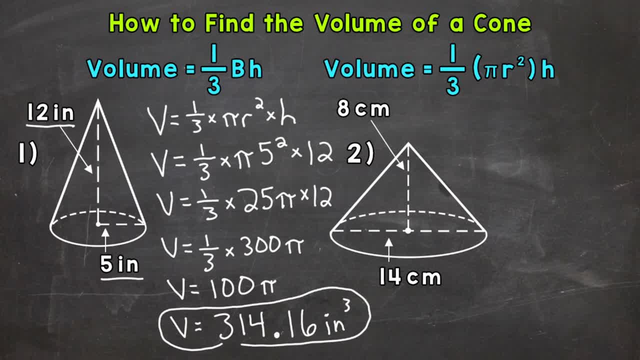 volume. So that's our final answer right there. So I want to explain why we multiply everything by one-third times pi. So I'm going to use the pi button on a calculator And I'm going to use the pi button on a calculator. 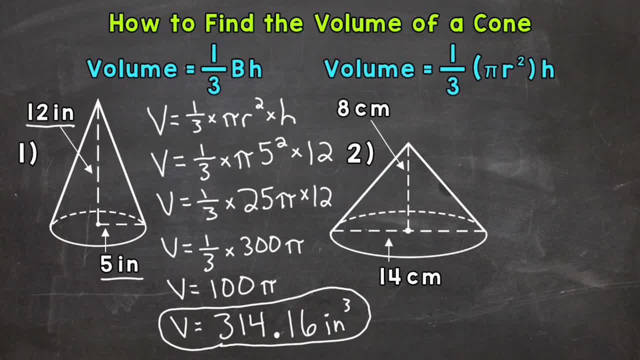 one-third If we take a cone and we put it in a cylinder with the same exact height and radius. let me try to draw this so we can picture it. So if we put this cone in a cylinder with the same exact radius and height, that cone is going to be exactly one-third the volume of that cylinder. 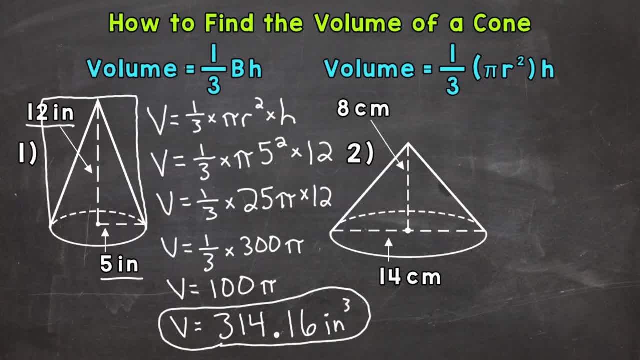 Pretty cool how it works out actually. Now, when we find the volume of a cylinder, we use the formula the area of the base times the height, So it looks really similar to this and this: The only thing we add in is the one-third, because, again, that cone is exactly one-third the size or volume of 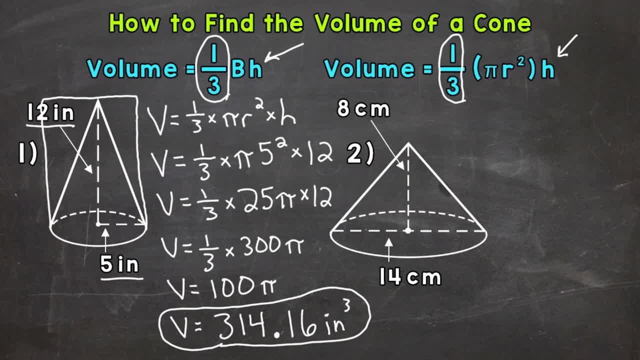 that cylinder. Let's move on to number two, where we have a cone with a given diameter for the base of 14 centimeters. We don't want the diameter, though. we want the radius, and remember the radius is half the diameter, so our radius will be seven. 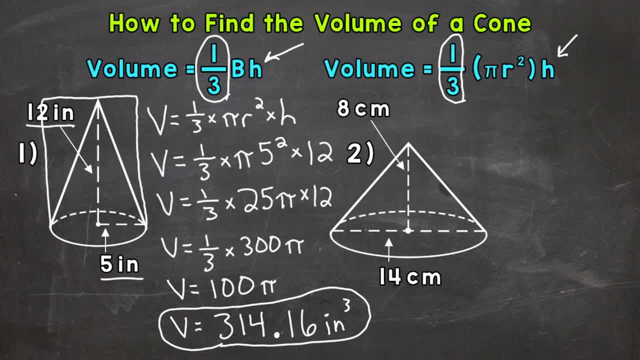 centimeters and then our height is eight centimeters. The first thing we do write out our formula. so volume equals one-third times pi, r squared times the height. Once we have that, we plug in. so volume equals one-third times pi. and remember our radius is seven because 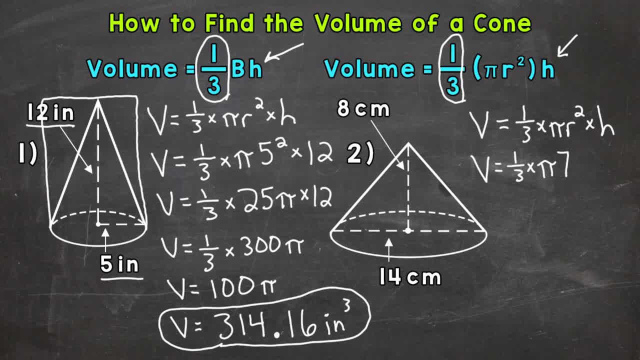 we're given the diameter and we need half of that for the radius. so seven squared times at the height of eight. Now we're ready to simplify this and break this down until we get our final volume. So next we'll do seven squared, so volume equals one third. We'll separate this by one third and we're going to do seven on the next circle, so five on the next circle, so the next three, and so so next. So if this is our final, So next size, Let's go back to one and put the 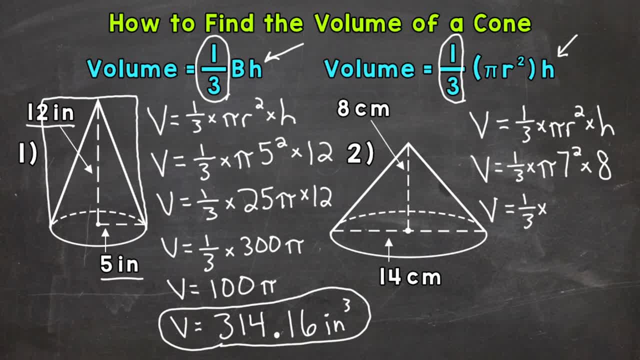 7 squared, that means 7 times 7, and gives us 49.. So we have 49 pi. That's the area of the base in terms of pi, And then multiply by the height of 8.. Our next step is going to be 49 times 8.. 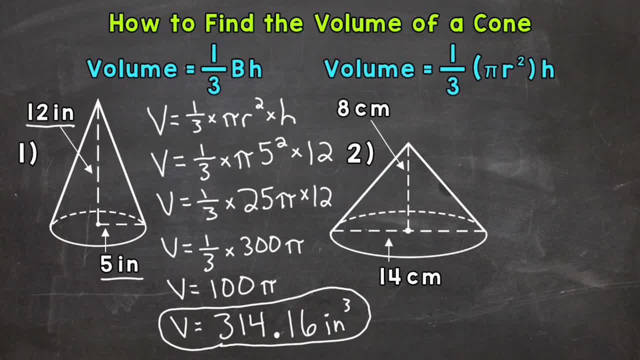 one-third If we take a cone and we put it in a cylinder with the same exact height and radius. let me try to draw this so we can picture it. So if we put this cone in a cylinder with the same exact radius and height, that cone is going to be exactly one-third the volume of that cylinder. 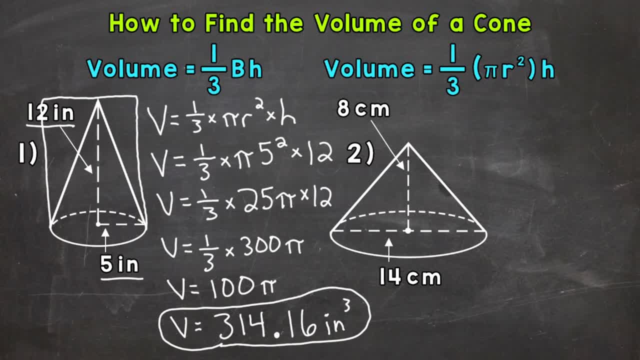 Pretty cool how it works out actually. Now, when we find the volume of a cylinder, we use the formula the area of the base times the height, So it looks really similar to this and this: The only thing we add in is the one-third, because, again, that cone is exactly one-third the size or volume of that cylinder. 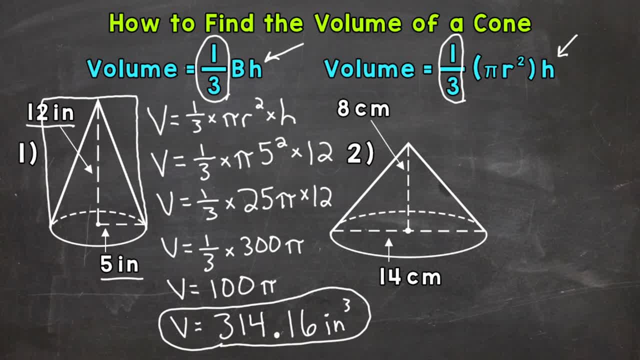 Let's move on to number two, where we have a cone with a given diameter for the base of 14 centimeters. We don't want the diameter, though we want the radius, and remember, the radius is half the diameter, so our radius will be seven. 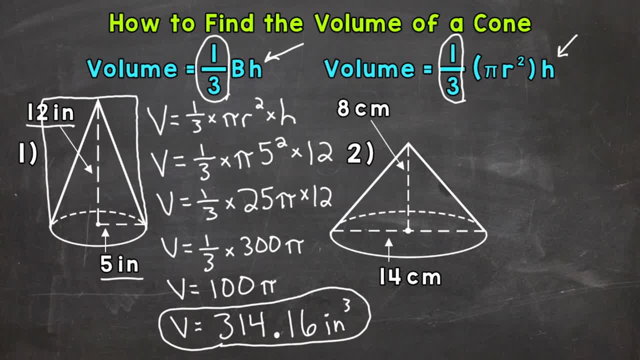 centimeters and then our height is eight centimeters. The first thing we do write out our formula. so volume equals one-third times pi, r squared times the height. Once we have that, we plug in: so volume equals one-third times pi. and remember our radius is seven because we're 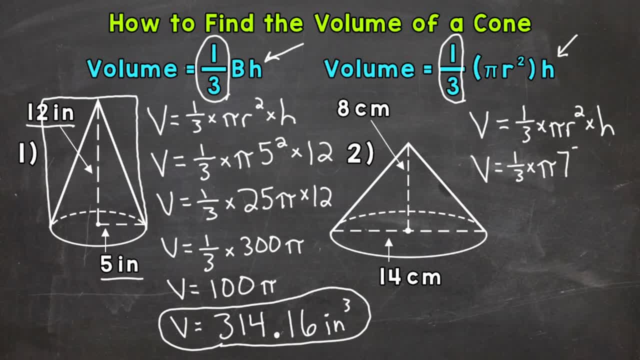 given the diameter and we need half of that for the radius. so seven squared times the height of eight. Now we're ready to simplify this and break this down until we get our final volume. So next we'll do seven squared, so volume equals one-third. 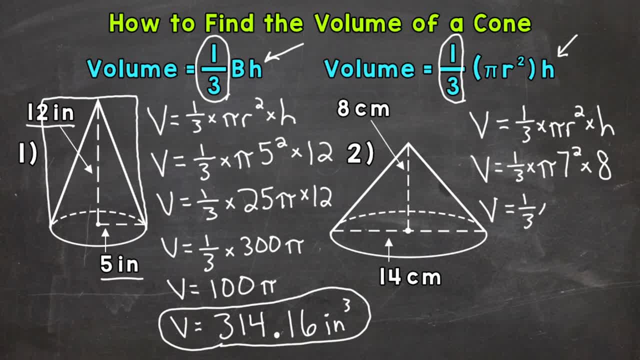 We'll do seven squared. that means seven times seven and gives us 49.. So we have 49 pi. that's the area of the base in terms of pi, and then multiply by the height of eight. Our next step is going to be 49 times eight. 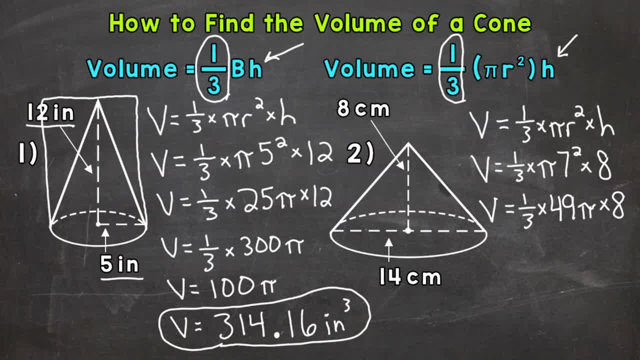 We don't have anything compatible with that 1 third that we can cross cancel. So 49 times 8 is our best option. So we'll end up with volume equals 1 third times 392 pi. Now we have to multiply 1 third by 392.. 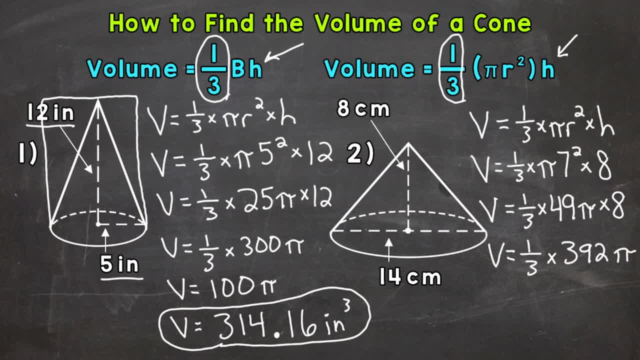 1 third and 392 are not compatible, meaning they don't work out nicely, like number 1, where we had 1 third times 300 and got a clean answer of 100.. So what we can do in order to simplify this to in terms of pi. 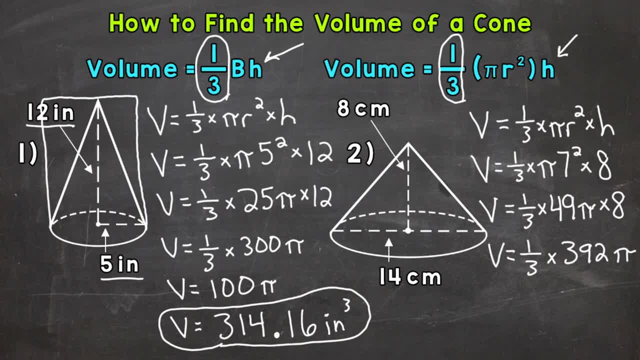 is to put it in fractional form: 1 third times 392 is going to give us 392 over 3.. So volume equals 392 over 3 pi, And that's our answer in terms of pi. But I want to back up and show you how I got 392 over 3,. 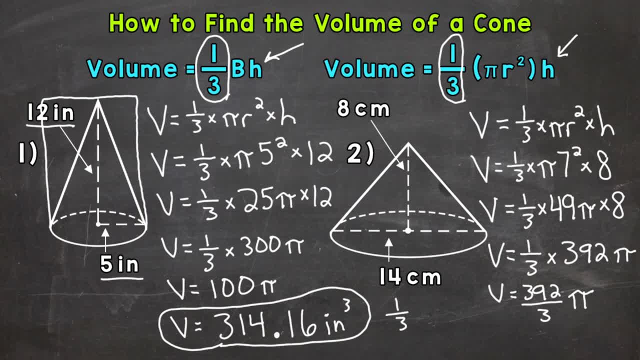 if you're unsure. So again, we did 1. third, and I'll try to squeeze this in over here- times 392.. Now, 392 is a whole number, so we can put it over 1 to put it in fractional form. 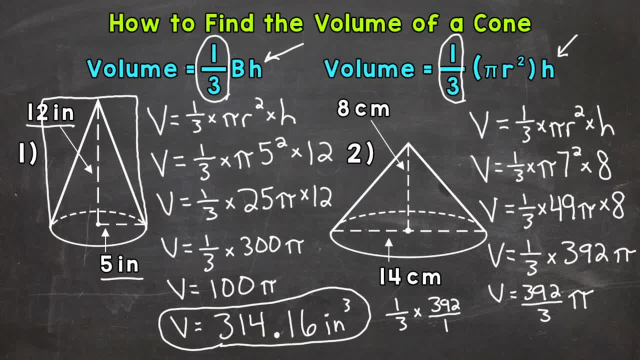 Now we can multiply. So in order to multiply fractions, we multiply straight across. So 1 times 392 gives us our numerator of 392, and then we do our denominator. So 3 times 1 gives us a denominator of 3.. 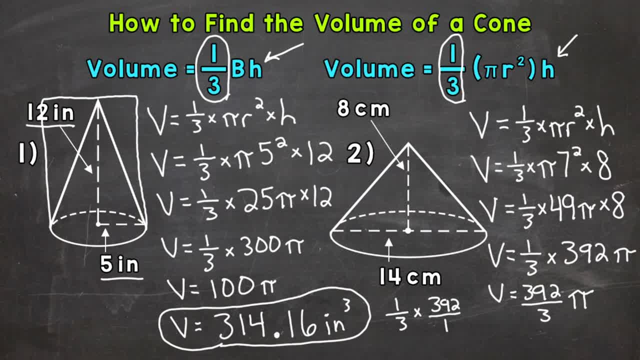 So again, that's our answer in terms of pi. So 392 thirds pi. Now we're going to calculate this and put it in decimal form by doing 392 thirds times pi. Now I'm going to use the pi button on a calculator. 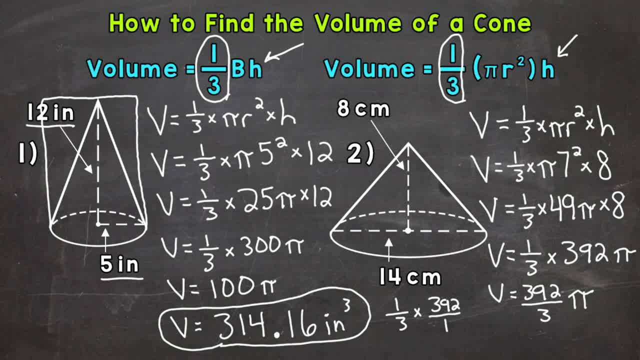 If you're using the approximate or rounded version of pi 3.14,, your answer is going to be slightly different than mine. So once we plug this in, we will get an answer of 410 and 50 hundredths. I'm rounding the decimal to the nearest hundredth. 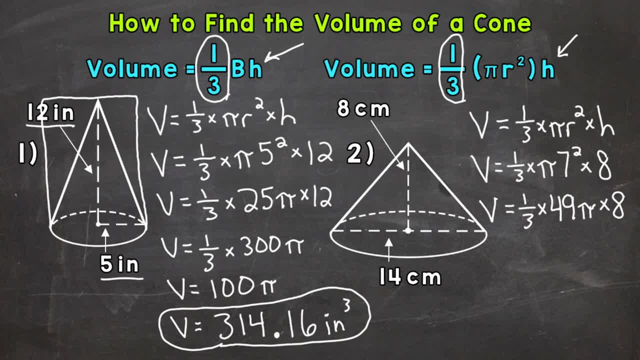 We don't have anything compatible with that one-third that we can cross cancel. so 49 times eight is our best option. So we'll end up with volume equals one-third times 392 pi. Now we have to multiply one-third by 392.. One-third and 392 are not compatible, meaning. 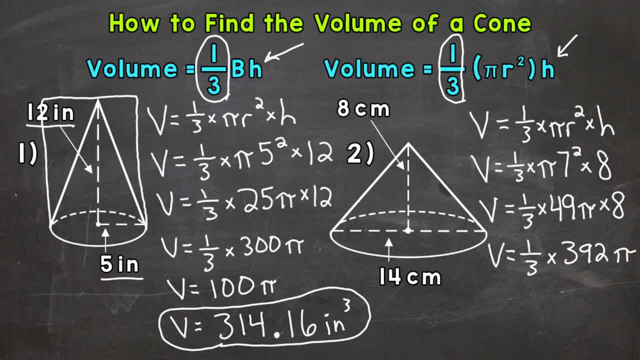 they don't work out nicely, like number one, where we had one-third times 300 and got a clean answer of 100.. So what we can do in order to simplify this to in terms of pi is to put our value in the fractional form: One-third times 392 is going to give us 392 over three, So volume equals 392 over. 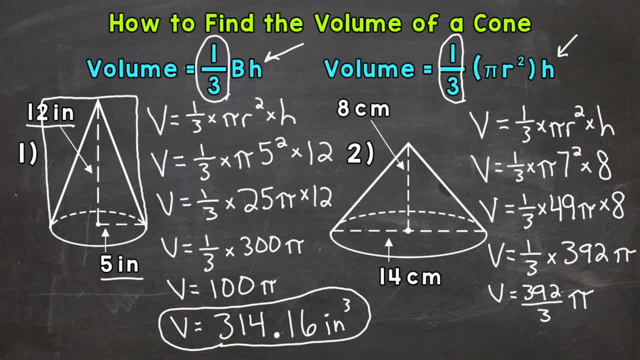 three pi, And that's our answer in terms of pi. But I want to back up and show you how I got 392 over three, if you're unsure. So again, we did one-third and I'll try to do it again. So we have. 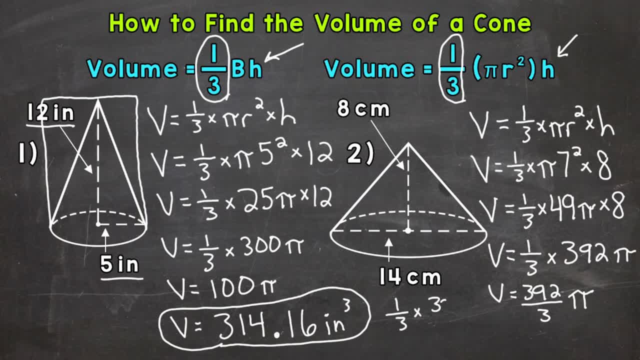 to squeeze this in over here: times 392.. Now, 392 is a whole number, so we can put it over one, to put it in fractional form. Now we can multiply. So in order to multiply fractions, we multiply straight across. So one times 392 gives us our numerator of 392, and then we do our denominators, So three. 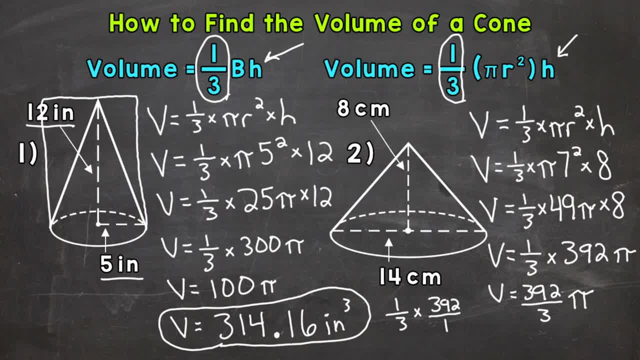 times one gives us a denominator of 392.. So again, that's our answer in terms of pi. So 392 thirds pi. Now we're going to calculate this and put it in decimal form by doing 392 thirds times pi. Now I'm going to use the pi button on. 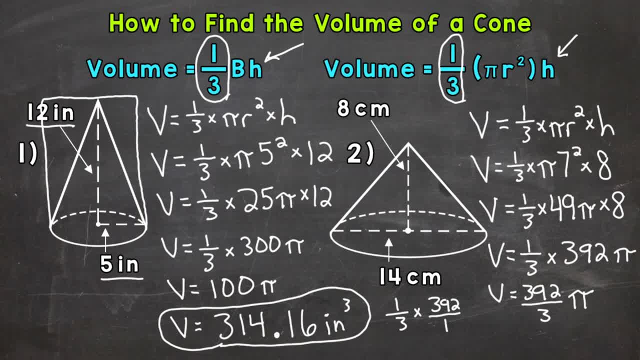 a calculator. If you're using the approximate or rounded version of pi 3.14, your answer is going to be slightly different than mine. So once we plug this in, we will get an answer of 392.. So we're going to get an answer of 410 and 50 hundredths. I'm rounding the decimal to the.